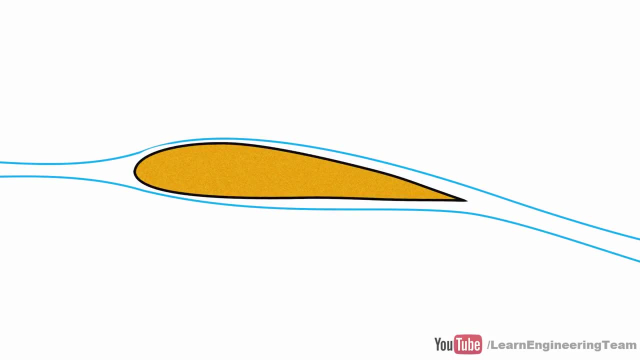 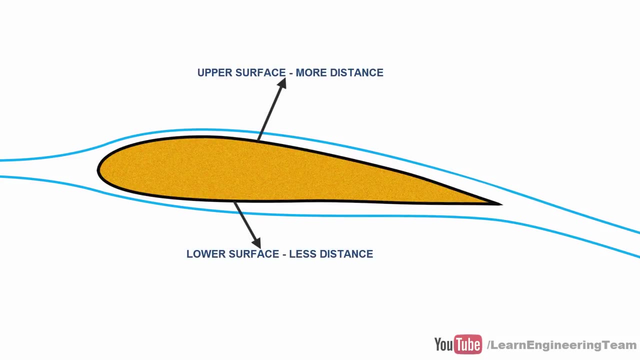 the video. First, let's see what is the argument that uses Bernoulli's principle: The particles on the upper surface should travel at greater distance than the particles on the lower surface, Since both particles should reach the trailing edge at the same time. 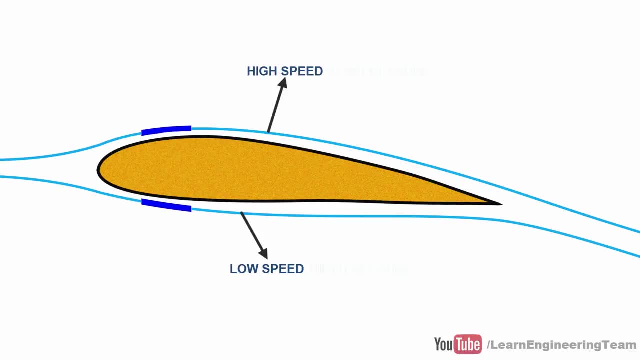 the upper surface particles should have more velocity than the lower surface particles. This means that, according to Bernoulli's principle, there is more pressure at the bottom bottom and less pressure at the top surface. The difference in the pressure generates lift. This argument, more specifically, is known as the equal time argument. 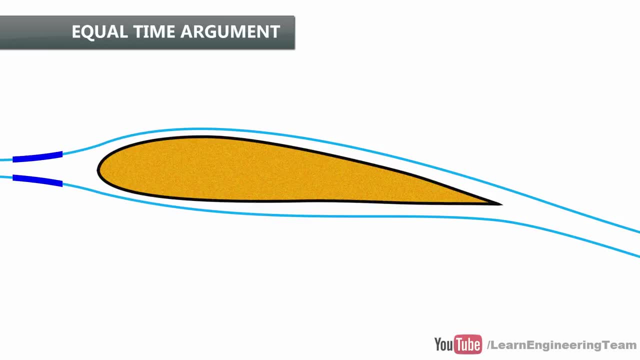 The equal time argument is a beautiful way to explain lift, but it's completely wrong. The first mistake pertains to how two particles starting from the same location reach the trailing edge at the same time. This is a completely absurd argument. There is no law in physics to support it. 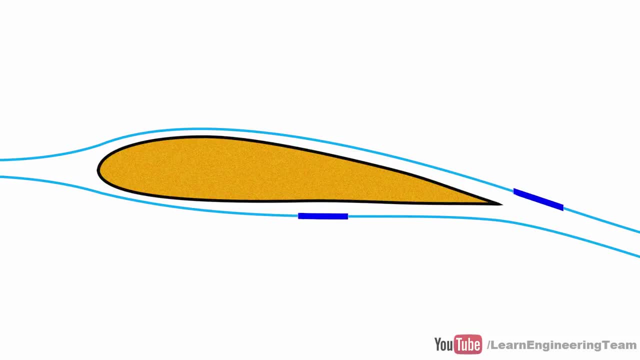 The two particles can leave for a completely different journey and may not meet in their lifetime. The second mistake is that you cannot apply Bernoulli's equation between two streamlines. Bernoulli's equation should be applied strictly along a streamline. Even after pointing out these mistakes, if you still support this widespread myth, just 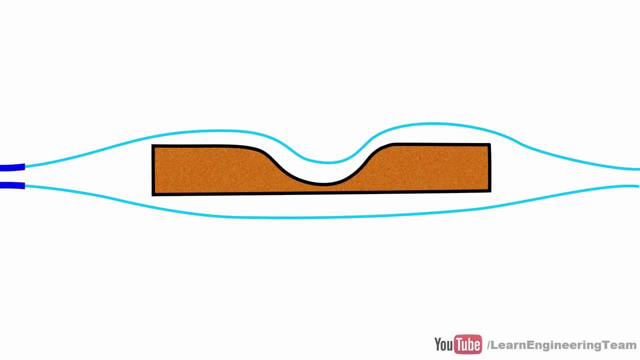 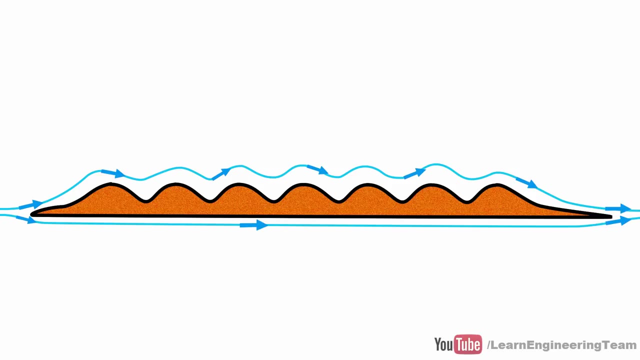 take a look at this shape. According to the equal time argument, lift is equal time. This surface should also produce a lift force, and this surface- The same argument- indicates that this should produce an incredible amount of lift. Bernoulli's equation is completely right. 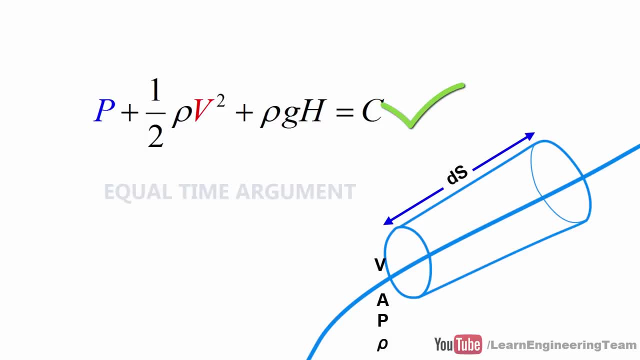 It is just Newton's second law of motion applied along a fluid streamline. Some people applied it incorrectly and caused confusion. Now we will investigate the second law of motion applied along a fluid streamline. The second law of motion applied along a fluid streamline. Some people applied it incorrectly and caused confusion. 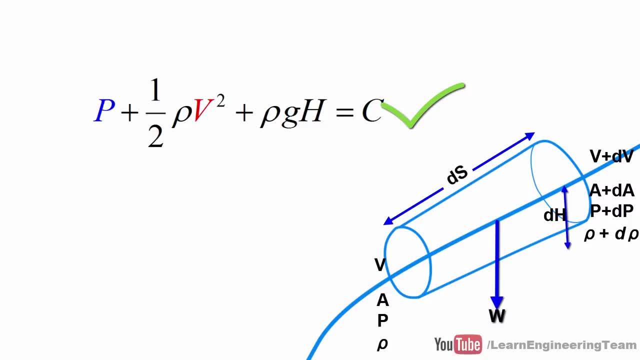 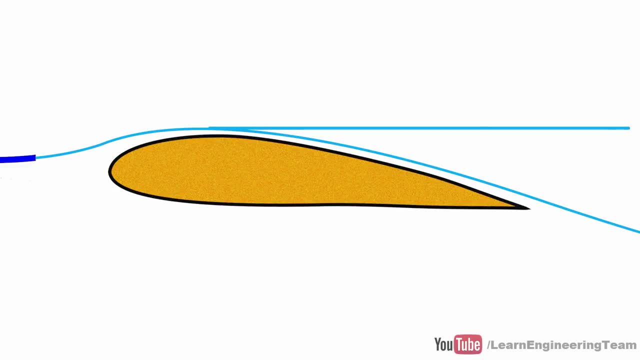 Some people applied it incorrectly and caused confusion. After änding one signal: Мы Gonzále ander mist landscaping the greenhouse maximum. by applying laws of physics correctly, The particle approaches the airfoil and takes a curve, as shown. But after the curve, why doesn't it move straight, as shown? 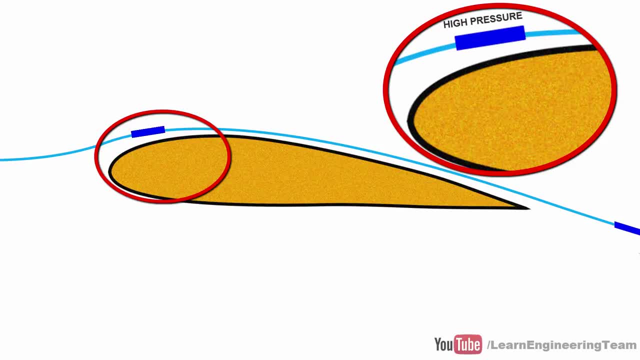 Examine this curved motion more closely. In order to take the curve, there should be more pressure at the top of the particle than at the bottom. This will supply the centrifugal force. This high pressure pushes the bands� Workshop Target gift離 in the travels. 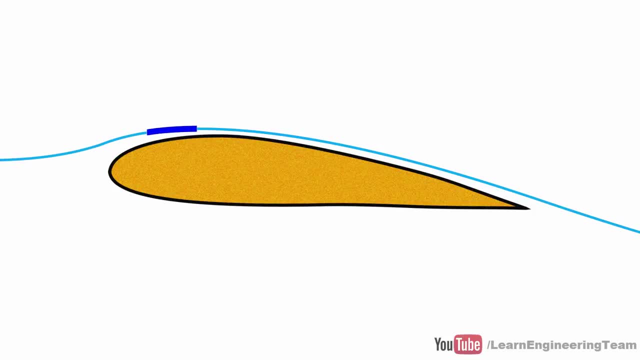 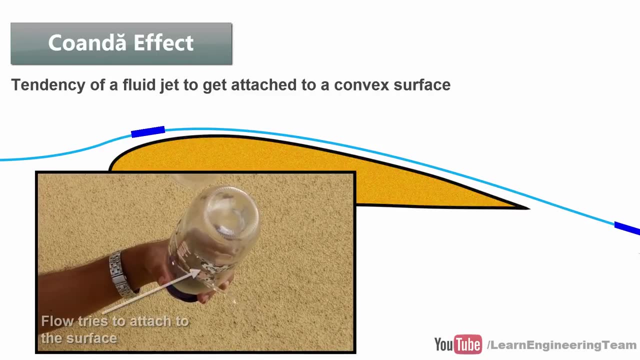 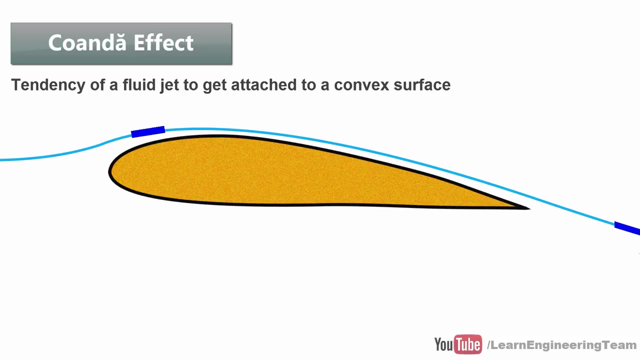 always attached to the airfoil. This effect is known as the Coanda effect. There is a simple experiment to demonstrate this fact. The flow gets curved at the bottom of the airfoil as well. A curved bottom surface will make the bottom flow also curved to a greater extent. 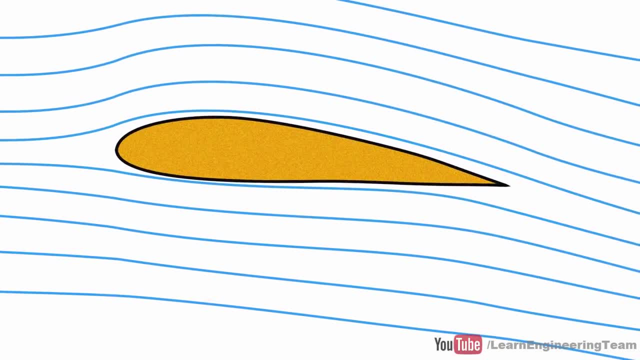 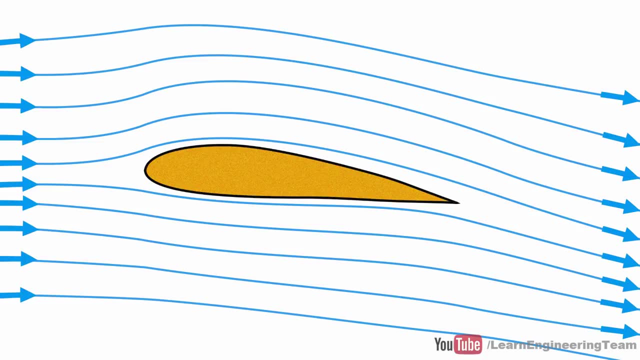 In short, the introduction of the airfoil makes the flow curved and deflected, and this curved flow is exactly what causes the lift. Let's see, Far away from the airfoil, the pressure is atmospheric, We know. in a curved flow the outside pressure should be larger. 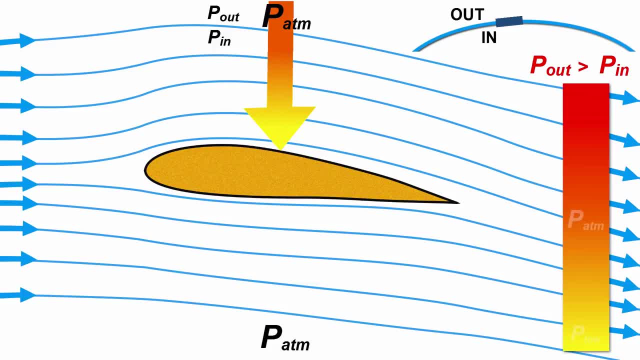 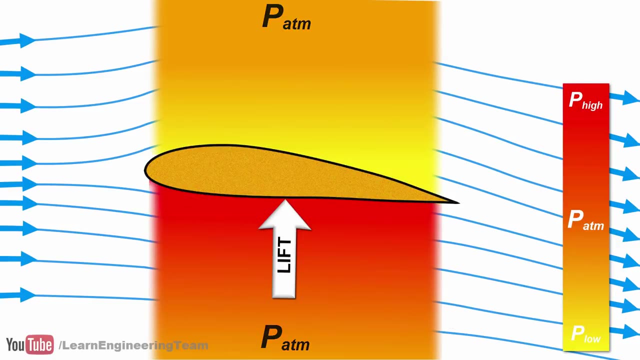 So at the top, the pressure will decrease as we move towards the airfoil. On the other hand, at the bottom and for the same reason, pressure should increase as we move towards the airfoil. This difference in pressure is what causes the lift. 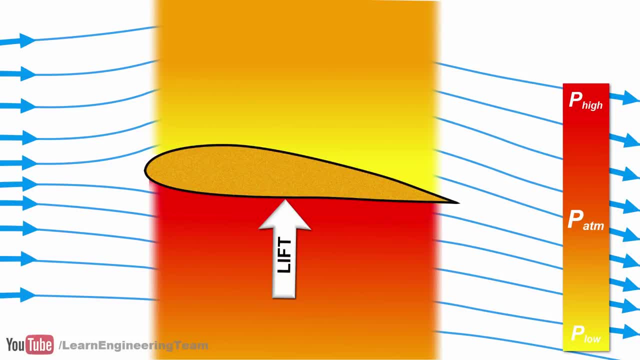 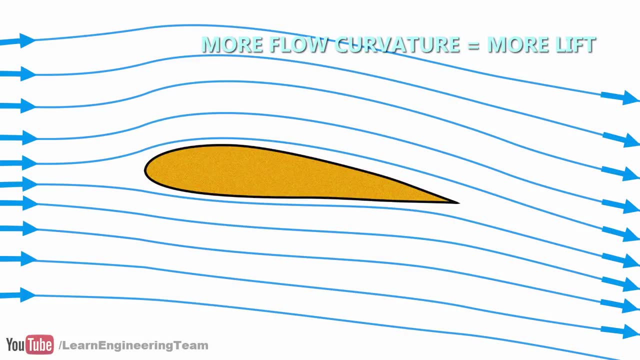 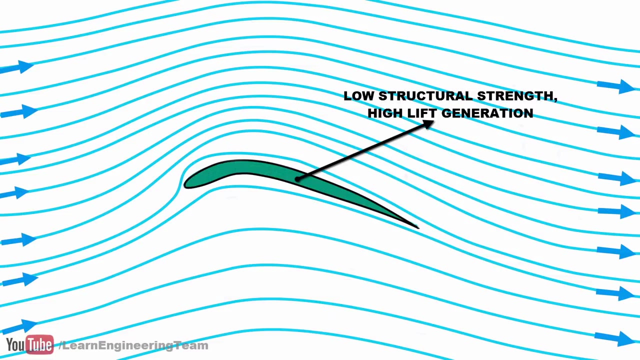 Basically, the introduction of the airfoil makes the flow curved. This curvature generates the pressure difference and the lift. This means that more curvature translates to more lift. But then why are airplane airfoils not shaped like this? The reason is to give structural support and a space for accommodating the fuel tank. 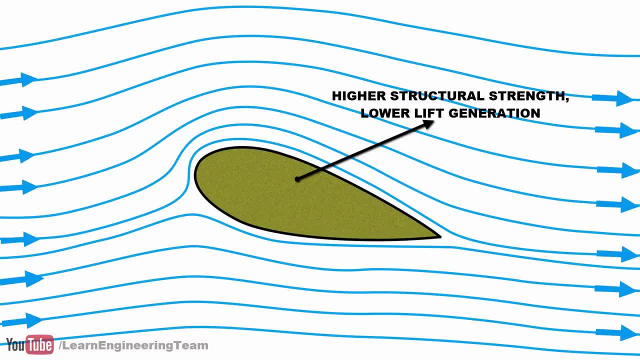 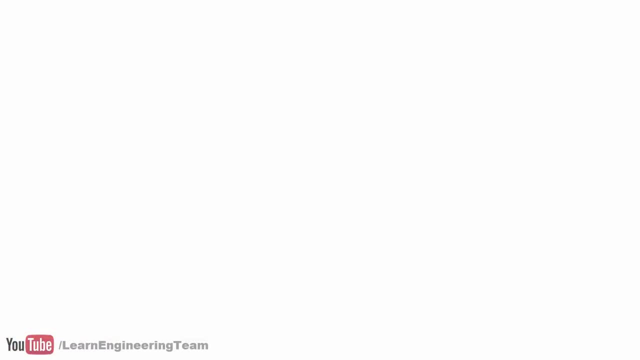 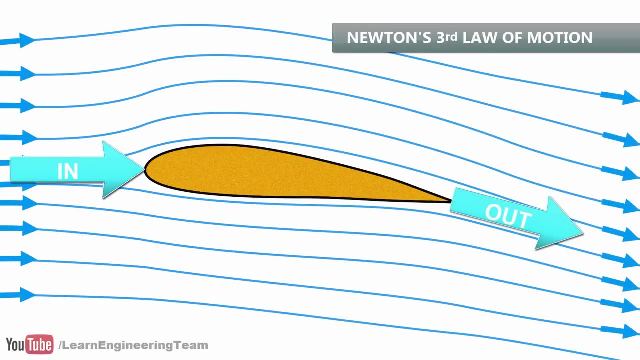 To do that, you need to know how the airfoil is built. Is there any fundamental law of physics that justifies the lift rather than this fluid mechanics-based explanation? Yes, Newton's Third Law of Motion. You can see that the airfoil deflects the flow as shown, or it pushes the flow downward. 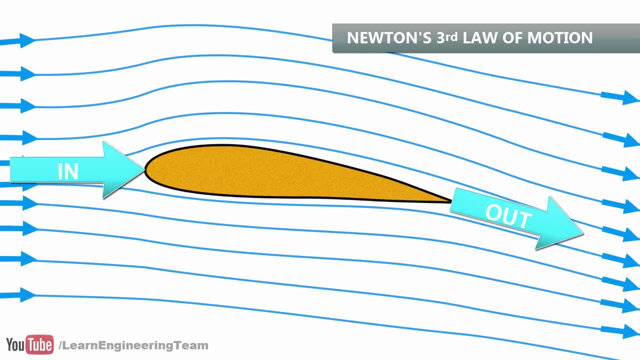 So, according to Newton's Third Law, the air also should push the airfoil in opposite direction with equal magnitude. This results in lift. In conclusion, the airfoil causes the lift, but it's not the same as what we've learned so far. The airfoil also pushes the airfoil in different directions with equal magnitude. This results in lift. The airfoil is also the same as the lift. It's the same as the lift. So according to Newton's Third Law, the air also should push the airfoil in opposite direction with equal magnitude.